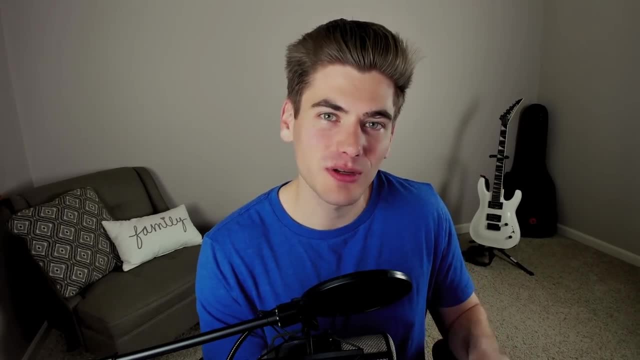 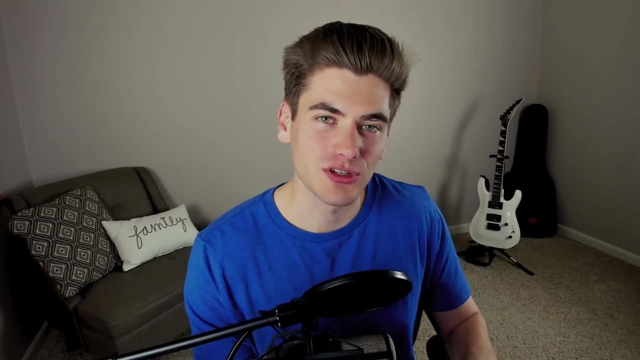 than normal JavaScript. If you don't understand why the things work in JavaScript, you're going to be really confused when you move to React, and some of the most important basics you need to learn are things such as scoping, so like where variables are scoped. you need to learn how. 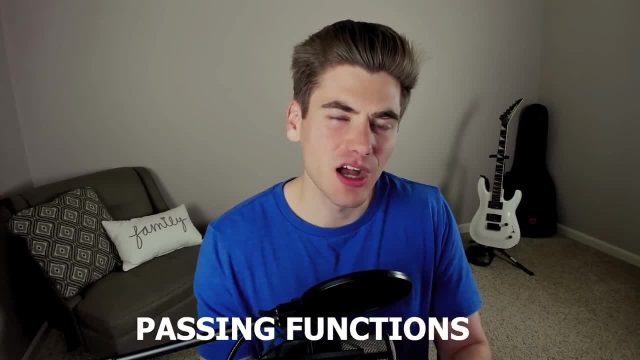 callbacks work and, most importantly, you need to learn how passing functions to other functions works. I know you probably already think you understand how passing functions to other functions works because you've done it with a computer. but if you don't know how to do it, 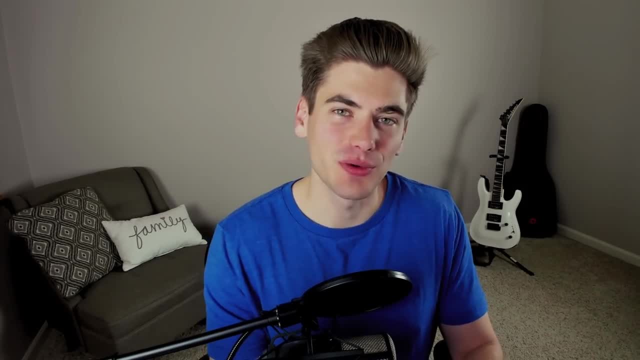 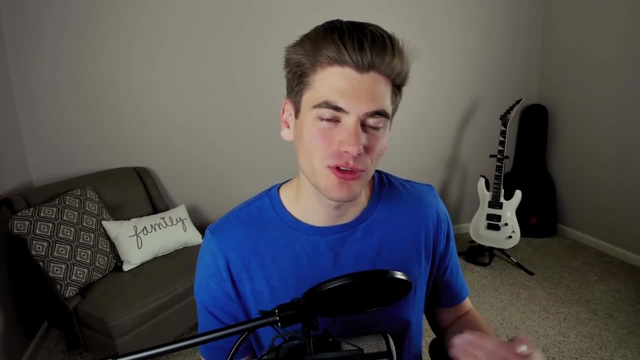 but if you don't really truly understand exactly what you're doing and why it works like it does, you're probably going to run into issues. when you start using event listeners in React- and that's probably the most common issue I see in React is people using functions inside event. 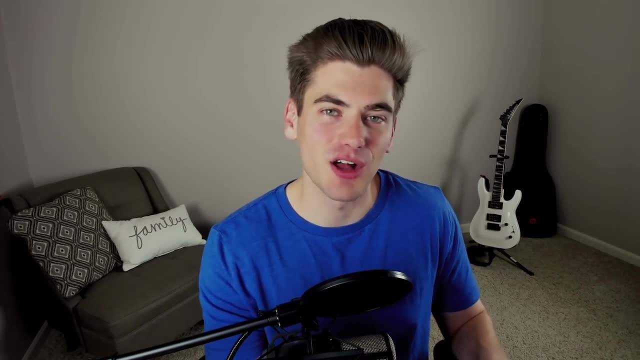 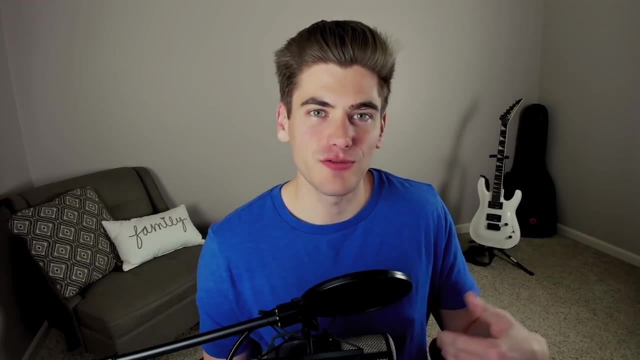 listeners the wrong way. so really make sure you understand how passing functions to other functions works. Another thing that's super crucial to React is understanding the difference between a reference and a value. You may know that if you create a const for an object called 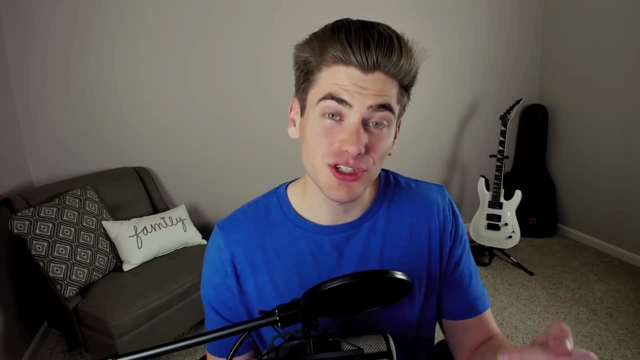 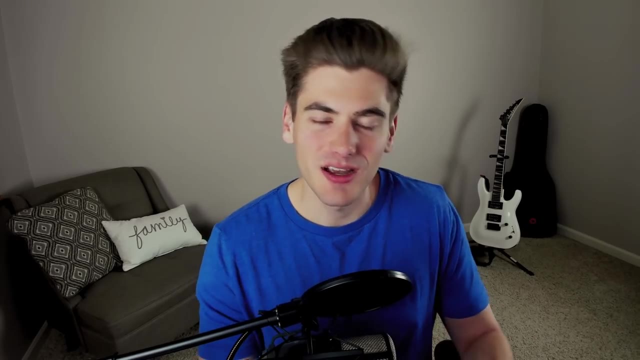 person. you set that person to like a object that has a name of Kyle, you can actually change the name property of that object to something else like Sally, even though the person object itself is a constant variable. that can't change. That's because objects and arrays and other things inside 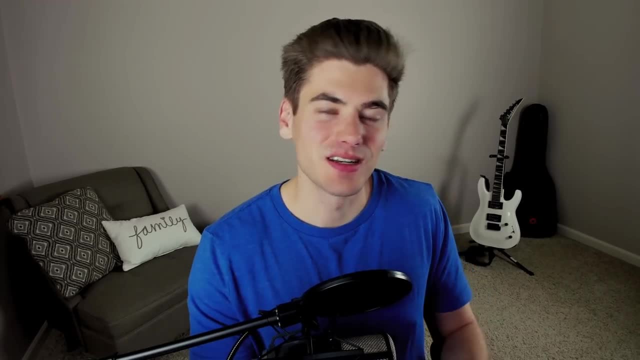 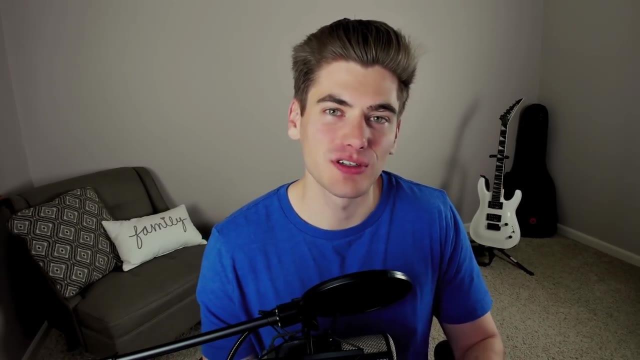 of JavaScript are handled as references, while things like strings and numbers and booleans- those are values, so you cannot actually change the value. If you want a little bit more of an in-depth guide on how references versus values work, I have a full video on it I'll link in. 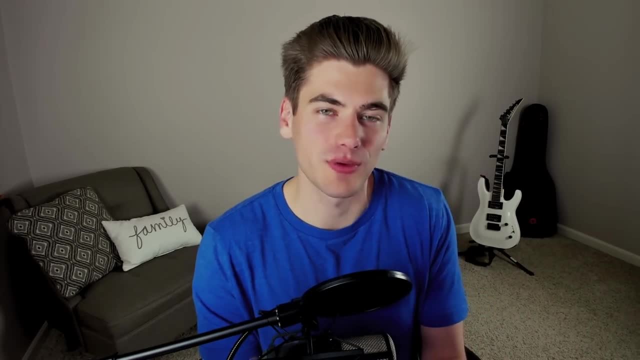 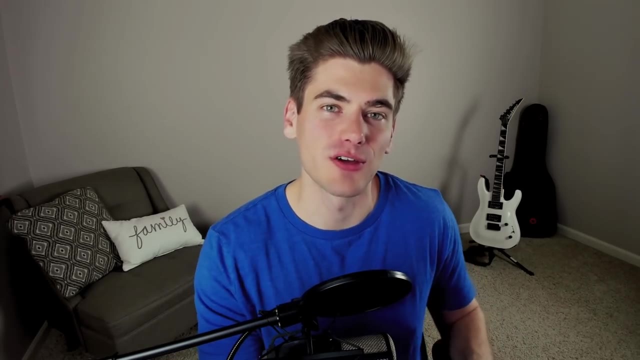 the cards and description for you, but this is a topic that's really, really important to React, because almost every single React hook- which is like the way you make logic in React- relies on understanding how references versus values work, and if you don't understand that, you're going to 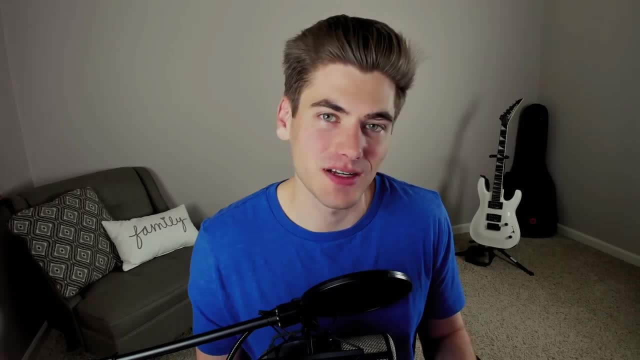 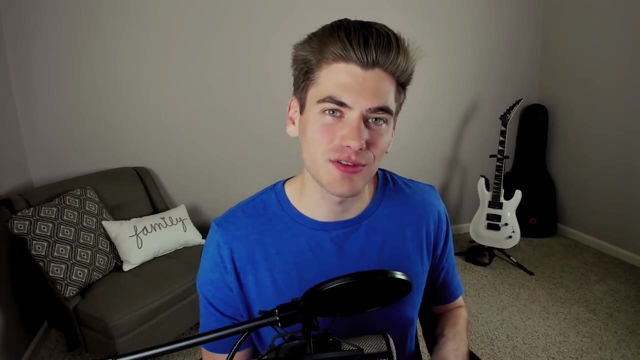 be completely lost and run into bugs that are seemingly impossible to fix. On that same topic, you need to understand the difference between the double equal sign and the triple equal sign and just how type coercion works inside of JavaScript is. again, that's something that React uses behind. 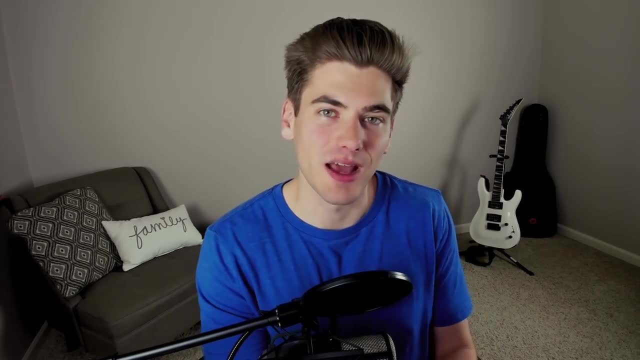 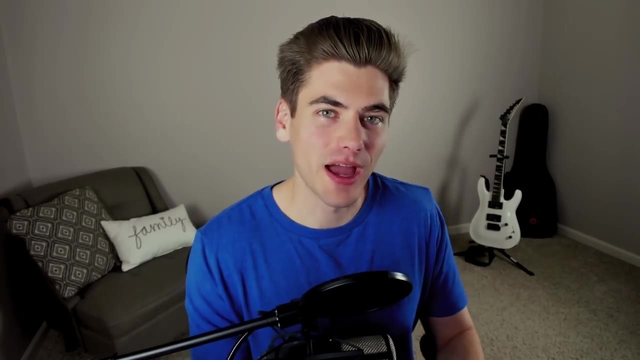 the scenes, and if you don't understand how that works, you're going to be really lost. looking at the React code, Another really important thing to know is things like advanced logic. so short circuiting is one of the biggest examples that you're going to see in React because, as you're 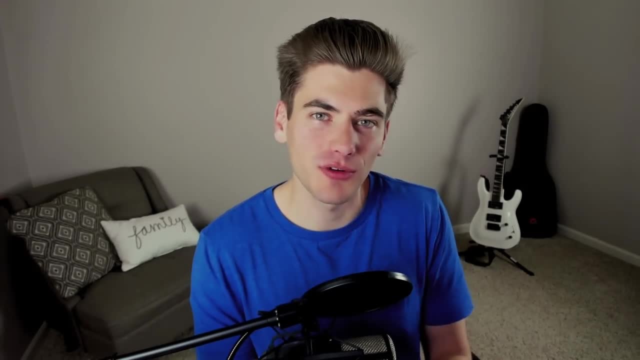 going to all the time see short circuiting. so you're going to see like a Boolean variable followed by like the double ampersand symbol and then some other code, and understanding how short circuiting works, how different if evaluations are done so like ands, ors and so on, how those 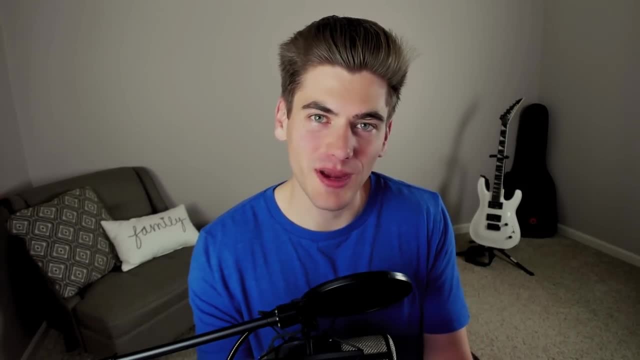 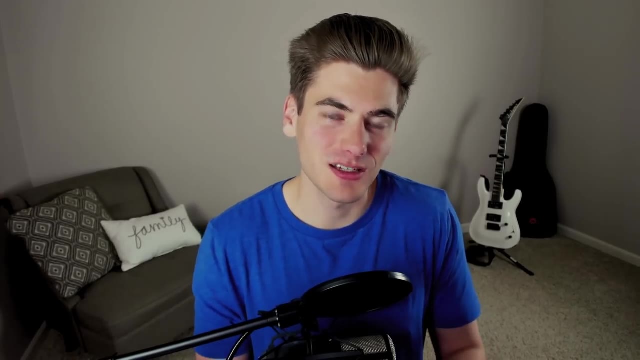 actually evaluate in order. it's super important because otherwise you're going to look at this React code. it's going to look completely foreign, but if you understand short circuiting it's going to make complete sense. Another really crucial topic to understand, especially when writing your 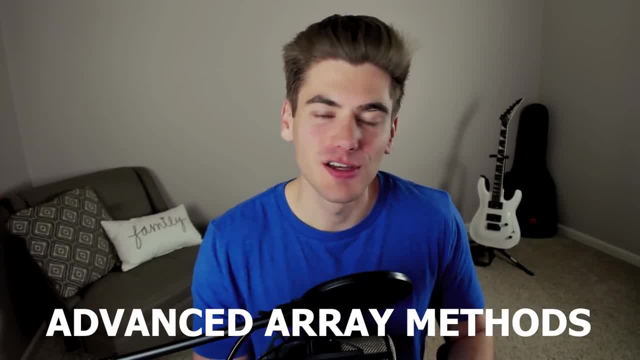 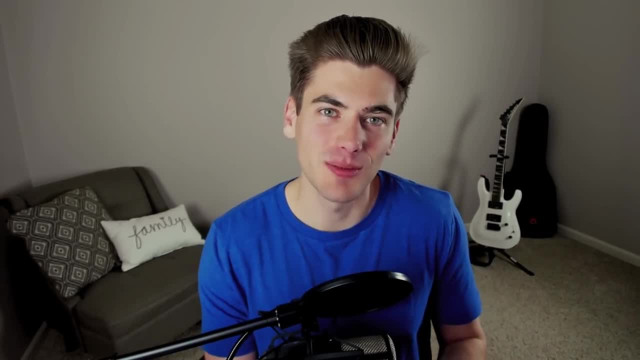 HTML in React is all the different advanced array methods, so things such as map and filter and sort of. you're going to see those all over React code for changing state and writing out your HTML. so if you don't have a really in-depth understanding of exactly how those methods work, 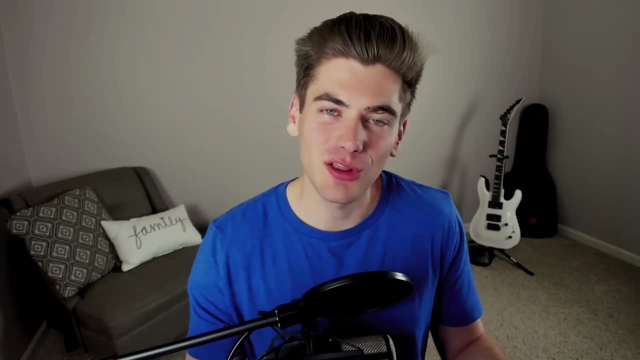 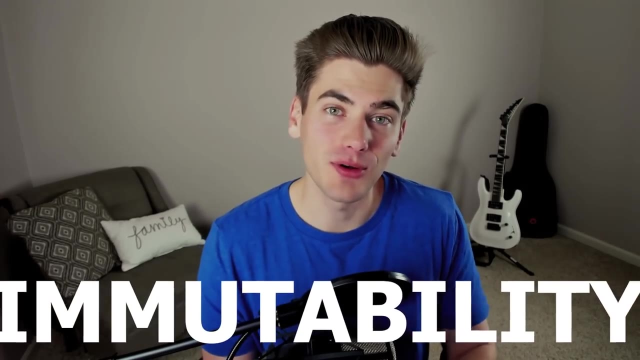 how they modify arrays and how they don't modify arrays. you're going to be completely lost again while writing out this React code And kind of speaking of the topic of modifying and not modifying arrays, understanding immutability and the idea of things being able to be modified, or 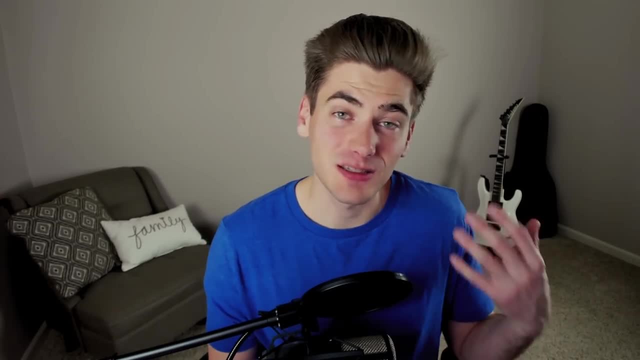 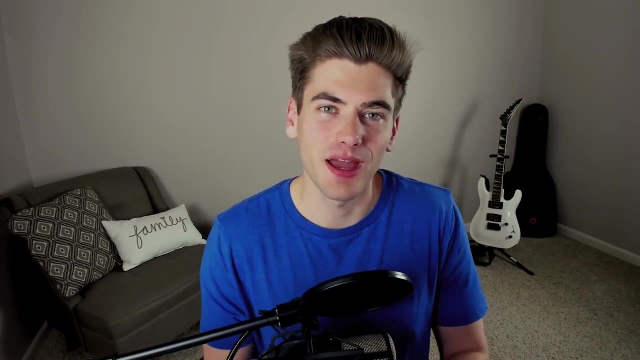 not modified is really important, because React has a lot of things based specifically on immutability. If you don't understand the concept of immutability, you're again going to be lost. Another thing you're going to see all the time inside of React is the idea of asynchronous code. 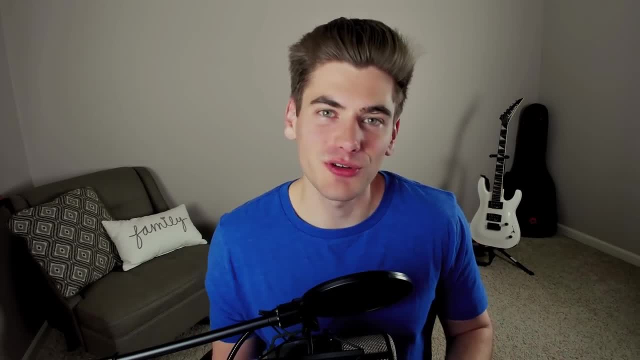 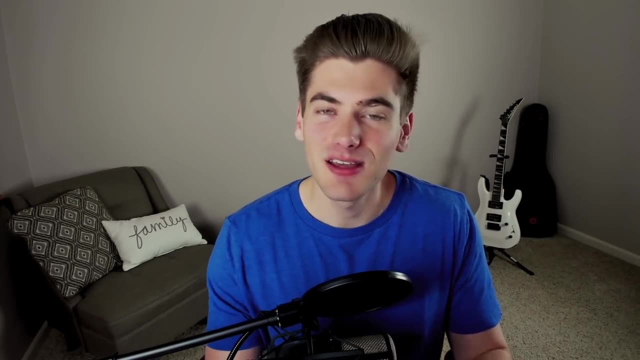 A lot of things in React run asynchronously in the background, so understanding not only how asynchronous code works and what it is, but also how you can write your own using things like callbacks, promises and async await, is really important, because that's just used all the time. 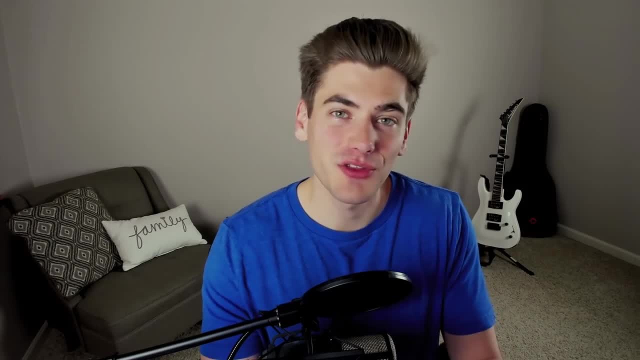 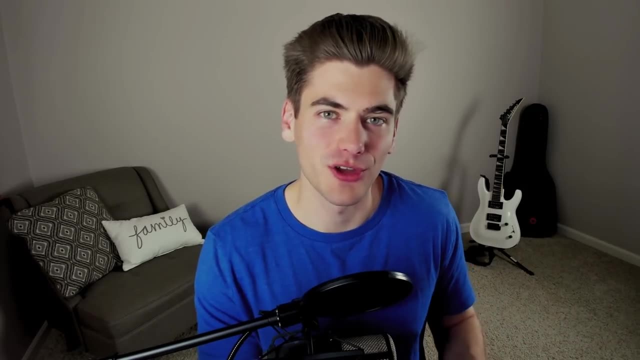 inside of React, especially with things like the useEffect hook. Another thing that's really important to understand is just the general concepts of modules. I know this is probably something you're most likely familiar with if you've written any amount of code. but knowing how to install node modules. you're going to be able to do that in a lot of ways. So if you're using a lot of code, you're going to be able to do that in a lot of ways. So if you're using a lot of code, 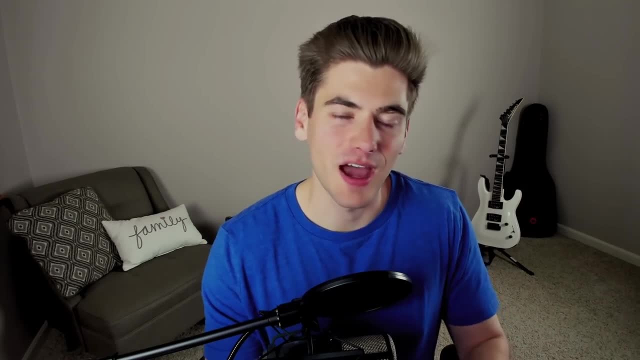 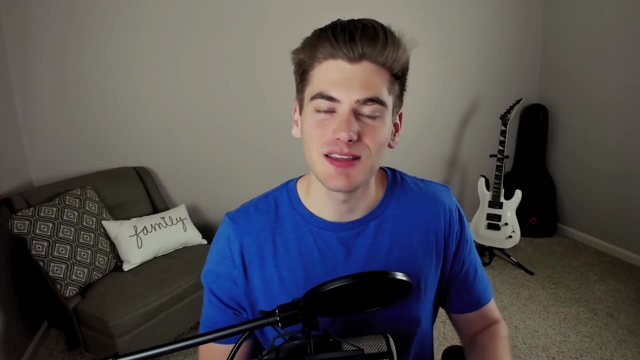 you're going to be able to install node modules, use and import them and use code like that and have modules inside of your own code. so breaking apart your code into different files that you import and export is really important to understand, because React is a huge ecosystem and it's all. 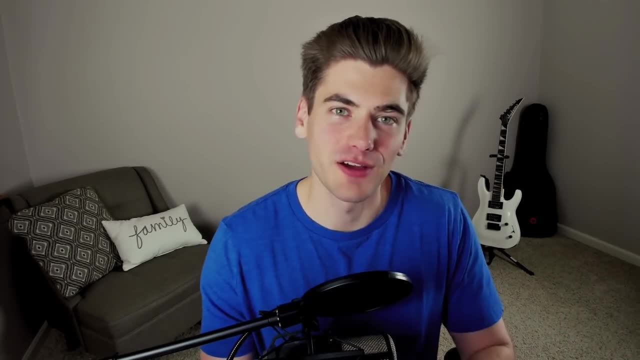 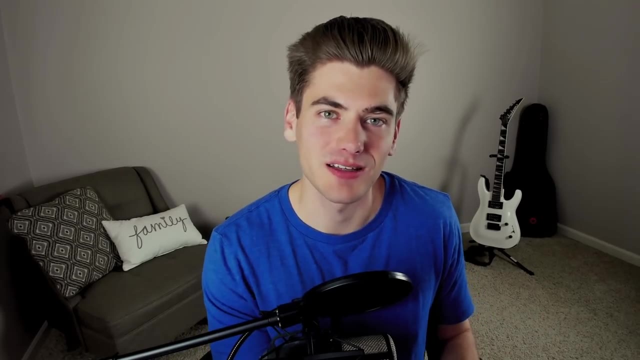 about making small components that you import and export into your different files as you need. So if you don't understand how to use module systems inside of JavaScript, you're not going to be able to use them inside of React, and they're not specific to React. I know a lot of. 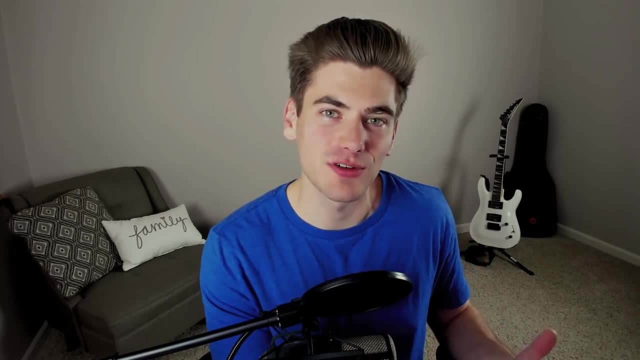 people think that import and export is React only because they never learn it in JavaScript. So if you learn it in JavaScript first, it'll be super easy to learn it in React. So if you learn it in JavaScript first, it'll be super easy to learn it in React. So if you learn it in JavaScript first, it'll be. 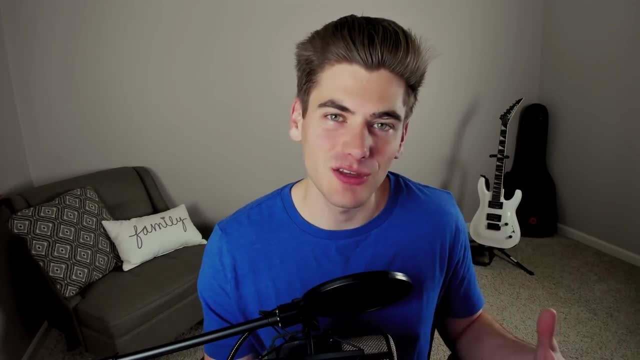 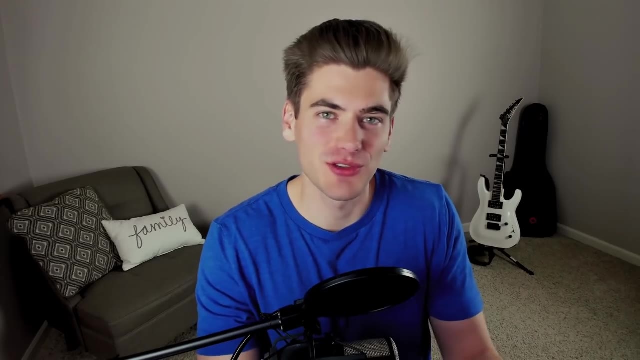 so much easier to implement it in React Also, kind of. the last main thing you need to learn is just the general concepts related to ES6.. ES6 introduced a ton of features like template string literals, destructuring the spread operator and so on, And making sure you understand exactly. 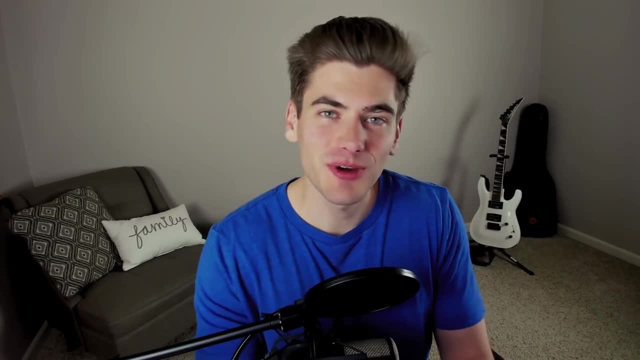 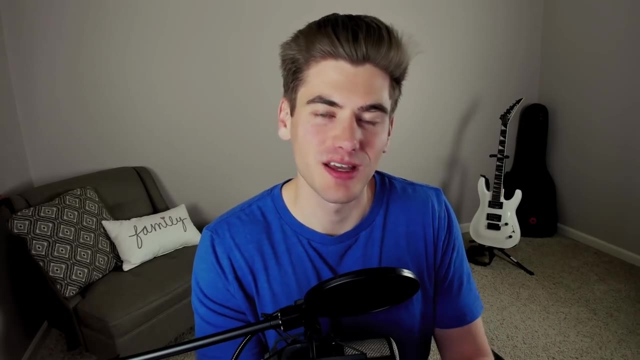 how all those different features work is crucial, because React uses pretty much every single ES6 feature And if you don't know how they work, you may think that they're like a special React only thing, when in reality is just plain JavaScript, And that's the important thing.